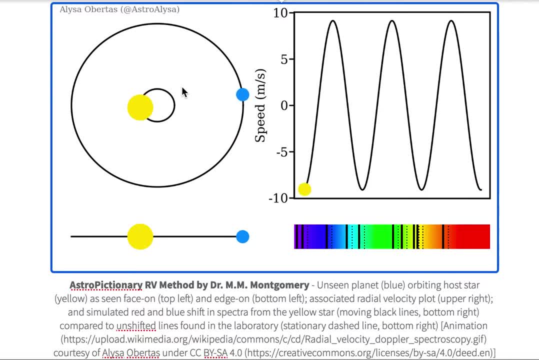 V for velocity. Here we have an animation by Alyssa Overdus. We're looking at a host star, which is the color yellow, and it is orbiting in the sky. In the edge-on view, we can see that the host star makes this wobble in the sky. It seems to wobble to the right, wobble to the left, and then back to the right. Because the star is wobbling or orbiting around a common point called the center of mass, we infer another object to be present in the system. We can only see the host star. We cannot see the exoplanet in the orbit. In this case, we have an exoneptunian system that's orbiting around its host star. Both the exoneptunian and the host star are orbiting the common point called the center of mass. 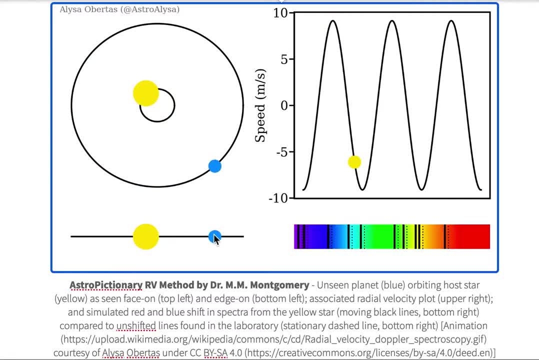 In the edge-on view, we can see the exoneptunian passing in front, and then going behind. 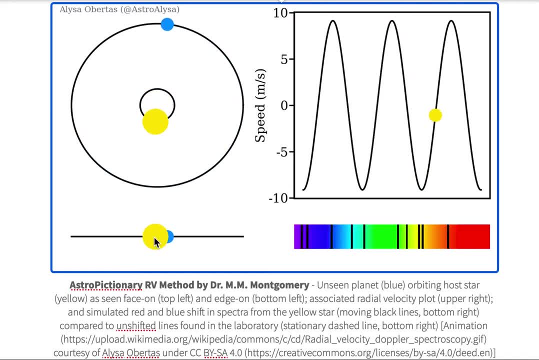 Passing in front, and then going behind. When we have an edge-on system like this, we are able to get spectra that show the shift in the wavelength of the observed star. 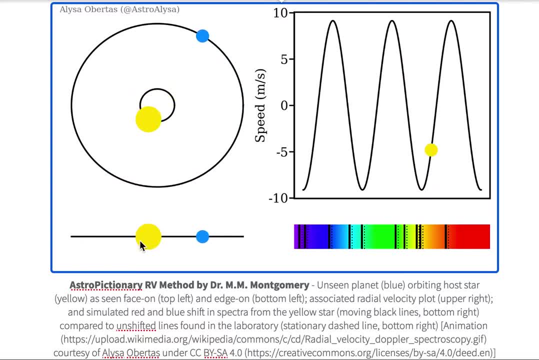 So we're focusing only on the star. We get the observed spectrum. Say we're getting the hydrogen-balmer lines and the sodium doublet. 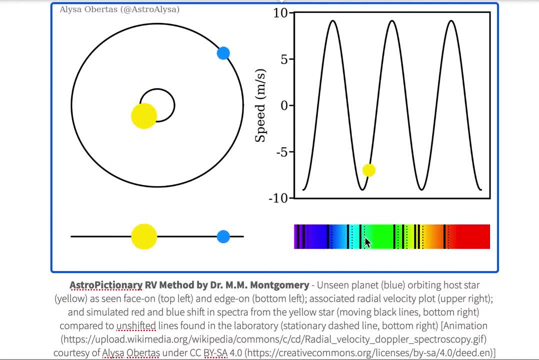 Observed spectrum is in the dark lines that we see. The background spectrum, the red, orange, yellow, green, blue, indigo, violet, is from the laboratory. And the dashed lines you see is the hydrogen-balmer lines and the sodium doublet as seen in the laboratory, those 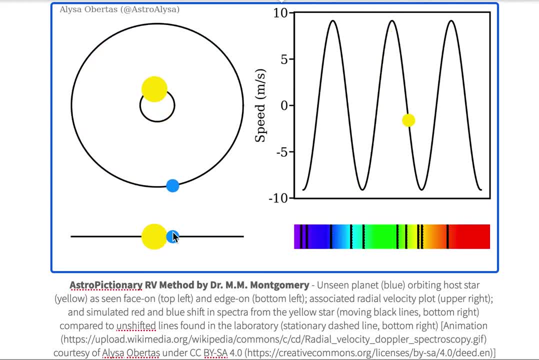 wavelengths that are seen in the laboratory. What we see from the host star is that the observed spectral line, let's say hydrogen-alpha, which I'm pointing to, has this red shift, and this blue shift. Notice the line is shifting towards the red side of the spectrum, 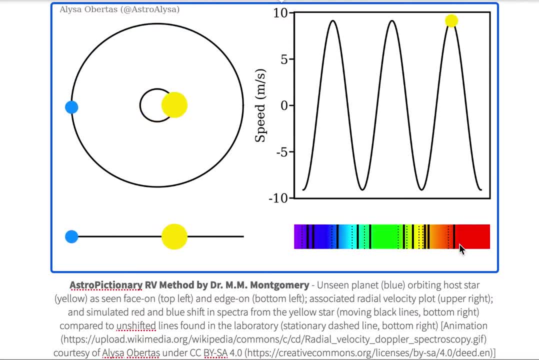 and then it shifts to the blue side of the spectrum. So the line has a red shift, a blue shift, a red shift, and a blue shift, and it keeps repeating. Because we see these shifting lines around the one line in the laboratory, we know that there must be something tugging on this star to make it make this wobble in the sky. 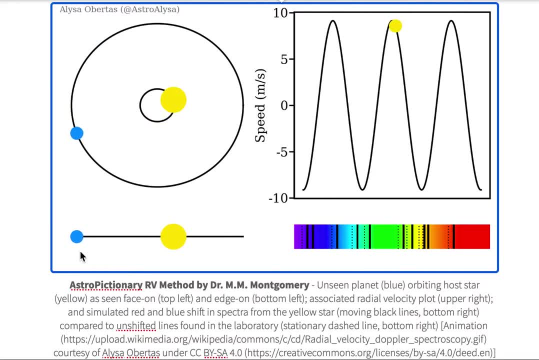 So we infer this exoplanet to be present. We can't image the exoplanet. We can only image the star. So we get the spectra from the star, and we see the spectral line shifting back and forth, which indicates that there is some kind of exoplanet orbiting around the host star. 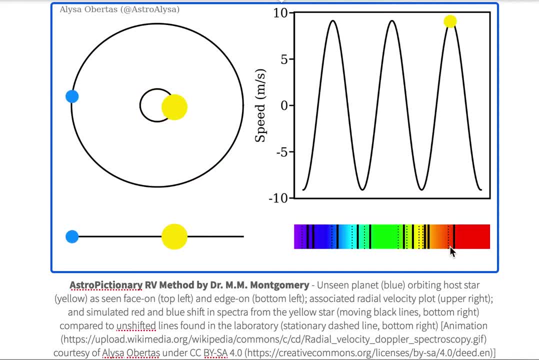 Now, the amount of shift is related to the speed of the star coming towards us or away from us. And we'll take a look at that next. 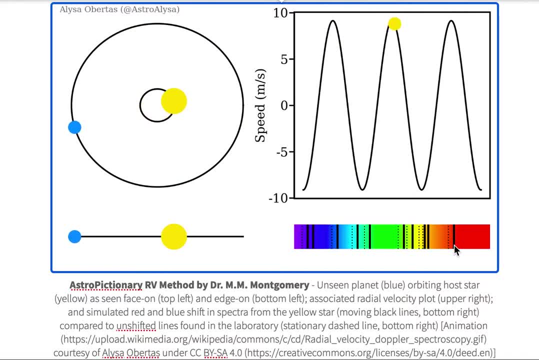 The maximum amount of shift is related to the speed of the star coming towards us or away from us. The maximum amount of blue shift or the maximum amount of red shift is related to the speed of 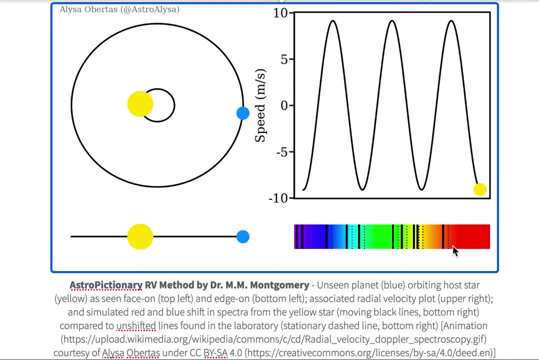 the star divided by the speed of light. The exact equation is the amount of shift from maximum red to maximum blue to the one that's in the center. So that delta lambda divided by the wavelength we find in the lab is equal to the speed of the star moving towards or away from us 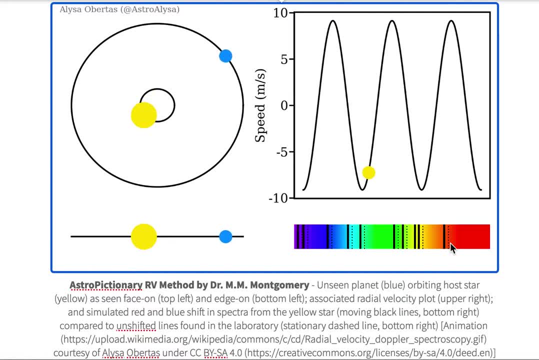 divided by the speed of light. We can take a look at this, in terms of the radial velocity or the speed over time. So we're looking at the speed of the star towards or away from us over time. And what we see is this star moving towards us and away from us, towards us and away from us. Towards us is negative numbers. Away from us goes to positive numbers. Negative numbers mean that the star is coming towards us or away from us. And so we can 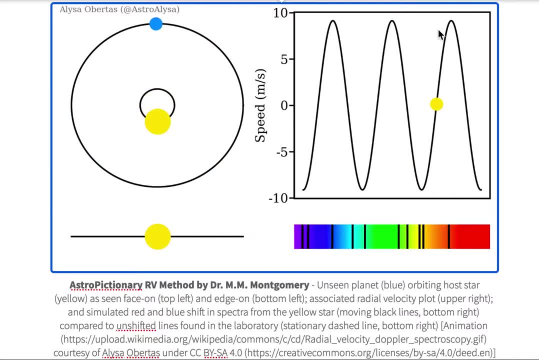 see that a positive values of negative is equal to positive ok that means energy and a positive тяж is equal to positive or goes along with this will say that we're looking towards us or away from us we call that a blue shift and positive numbers means the star is going away from us we call that 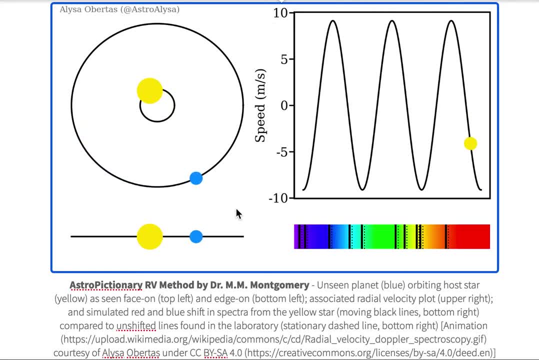 a red shift. See we got a red shift lines go to red we got a blue shift lines go to the blue we're 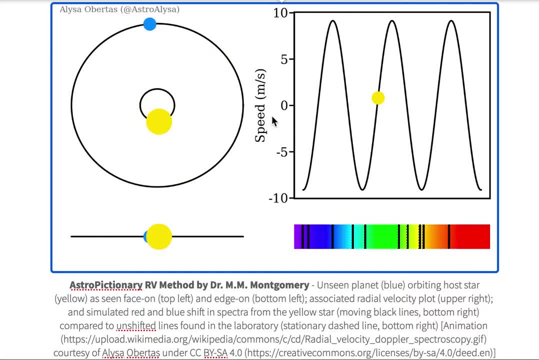 going to a red shift lines go to the red, coming towards us we got a blue shift. So we're looking of the star over time 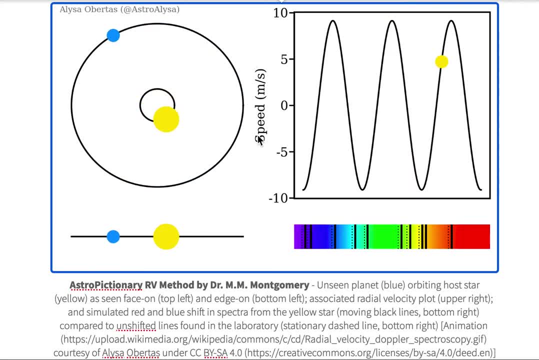 star divided by the speed of light. And that's what we have here on the left-hand side. So this is how qualitatively we determine the radial velocity method. Now radial velocity means that